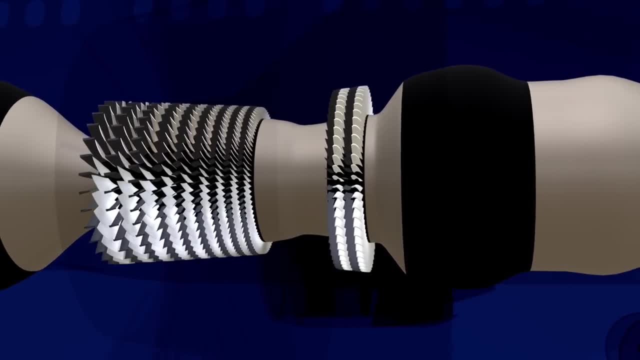 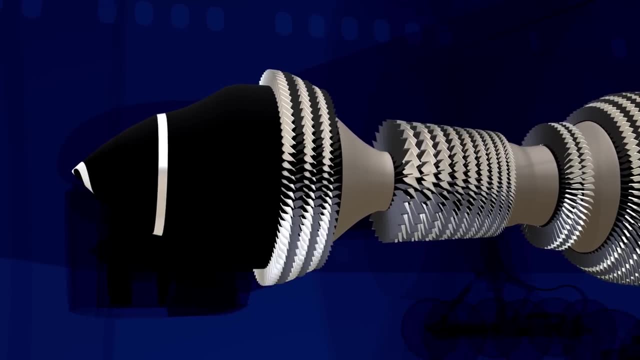 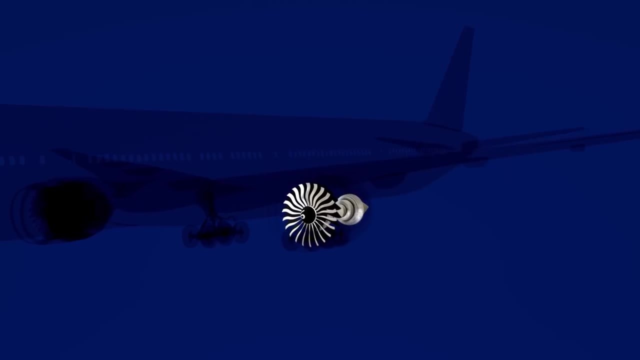 And two stages of high-pressure turbine. The N1 shaft has six stages of low-pressure turbine, Four stages of low-pressure compressors And ahead of them is the massive fan. Before we look at more engine components, let's do the aircraft configuration for engine start. 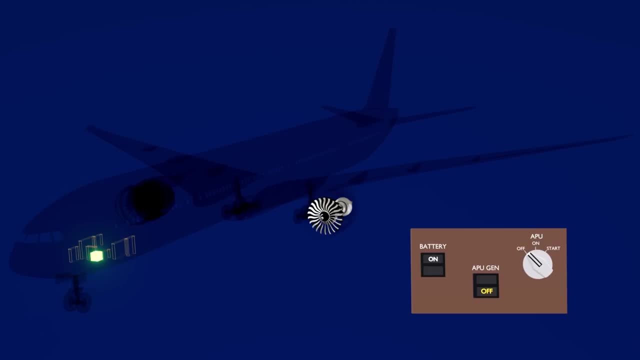 First the battery switch. Battery provides limited power, good enough to start the APU, A small engine in the impenage of the aircraft. Rotate the APU start switch, hold for a second and release. The APU is online now we can use the APU generator. 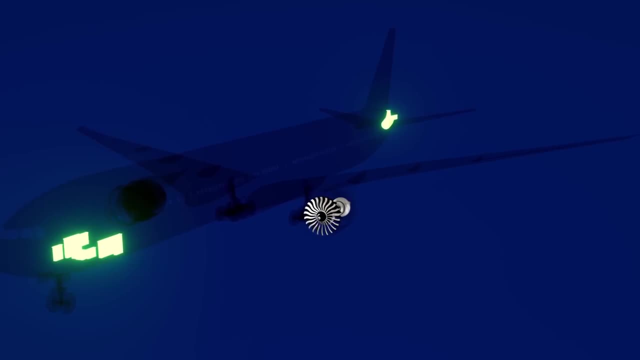 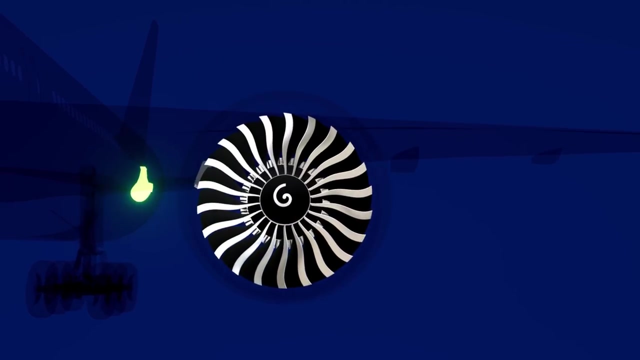 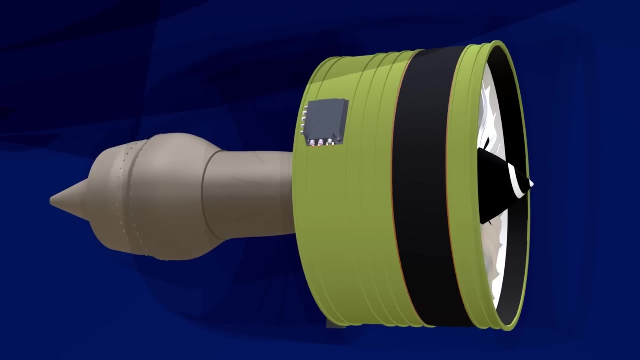 Selecting the generator switch establishes full electrical power of the aircraft. During engine start, electrical panels will provide power to the electronic engine control installed on the engine fan case. The APU will also provide the pneumatic power to start the engine. 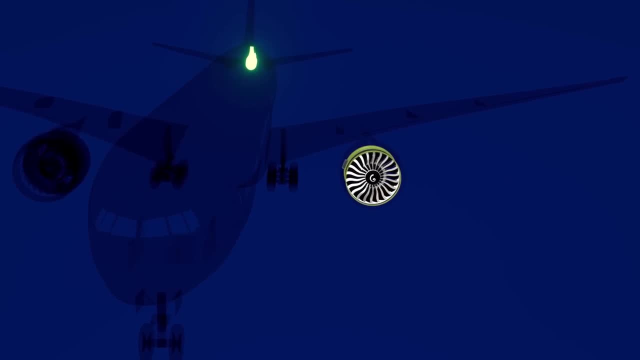 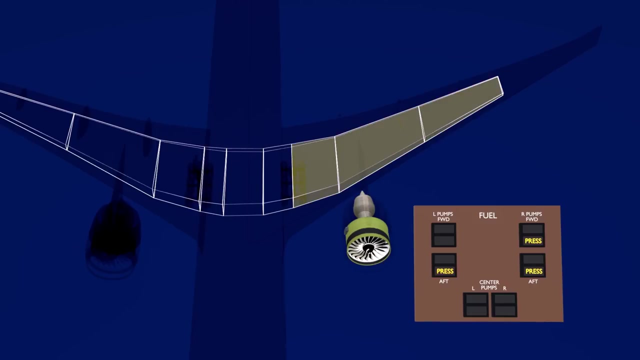 Make sure the bleed switch is in auto position. Next, the Fuel Panel selections. The APU will also provide the pneumatic power to start the engine. Make sure the bleed switch is in auto position. Next, the fuel panel selections. We only require fuel from the left main tank, so select the two left tank pump switches. 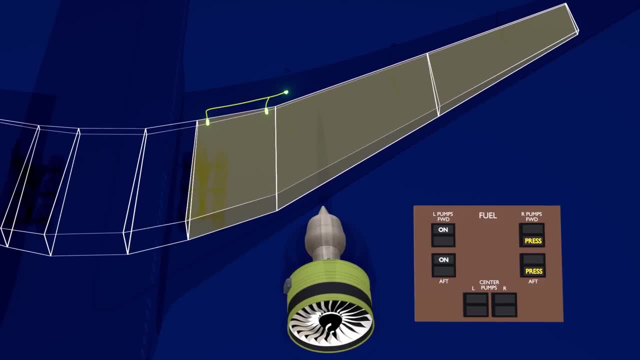 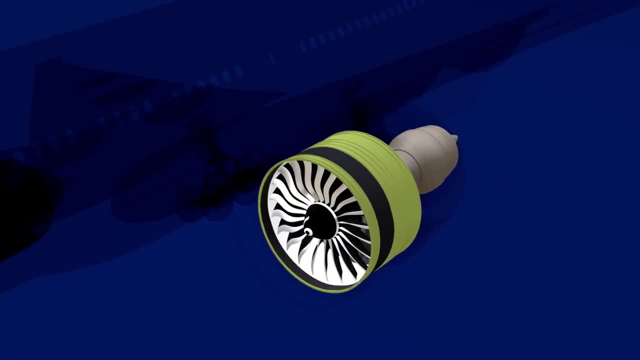 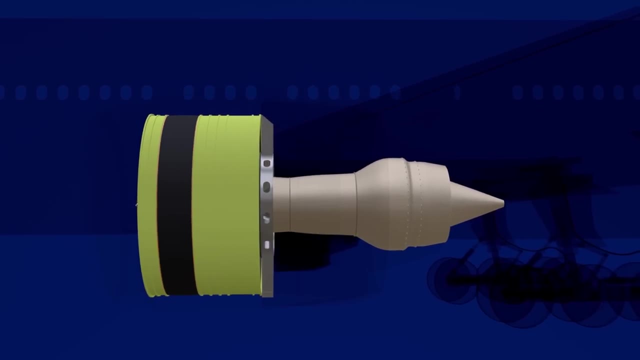 Two boost pumps inside the fuel tank transfer fuel to the engine. spar valve in the working compartment in the left, meaning hogging pump in the wing aft spar section. Aircraft configuration is complete. let's attempt an engine start On the engine. the pneumatic pressure reaches the start valve. 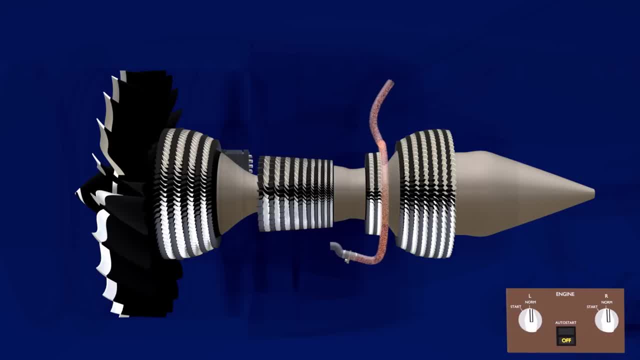 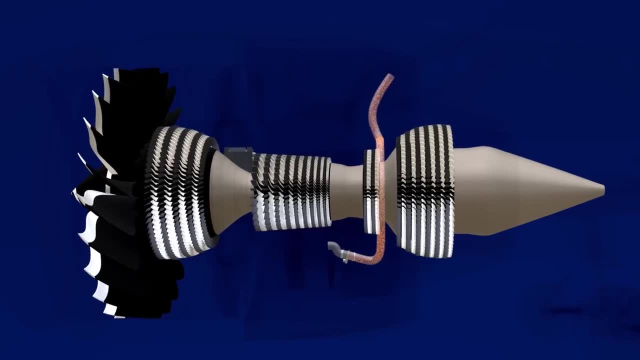 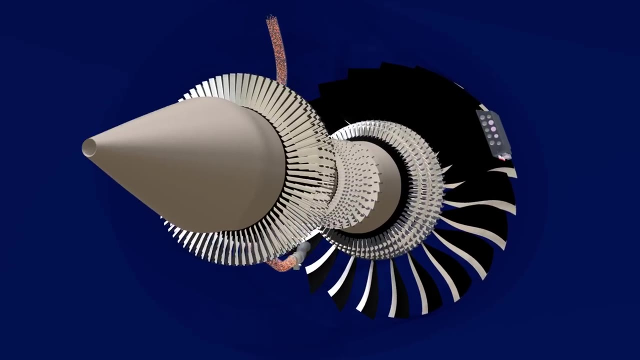 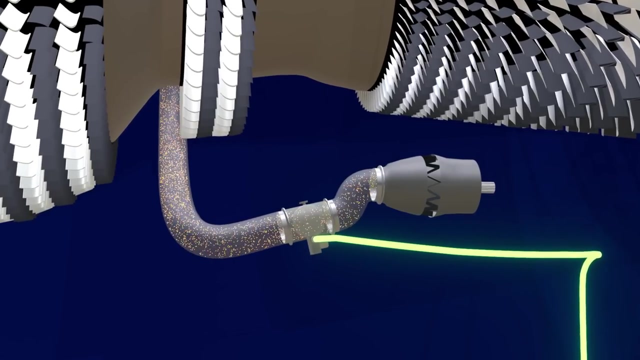 777 has an auto start feature. when used, the EEC takes over the entire engine start operation. Now turn the engine start, switch to start position. EEC gets the start signal and power to operate. EEC commands the start valve to open. the pneumatic pressure reaches the air starter. 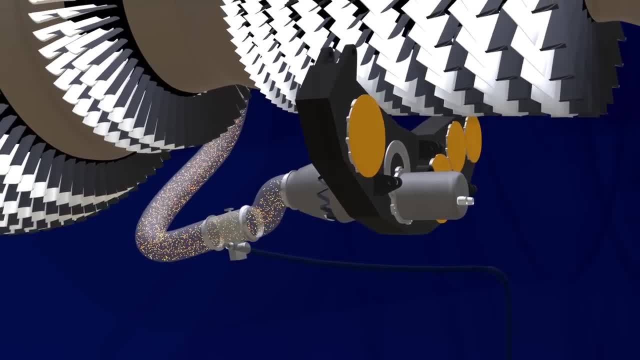 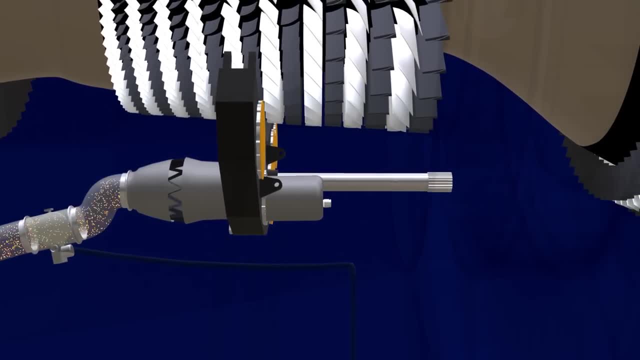 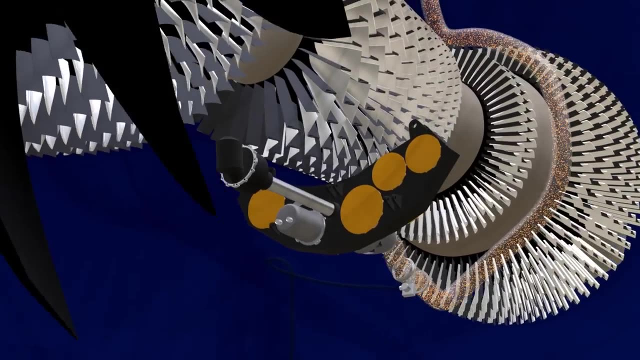 The air starter drives. the accessories- gearbox, Several torque requiring components are mounted on the gearbox. One of them is the horizontal drive shaft which connects to the transfer gearbox. The transfer gearbox changes the axis of rotation and, with the help of a radial drive shaft, rotates the N2 shaft. 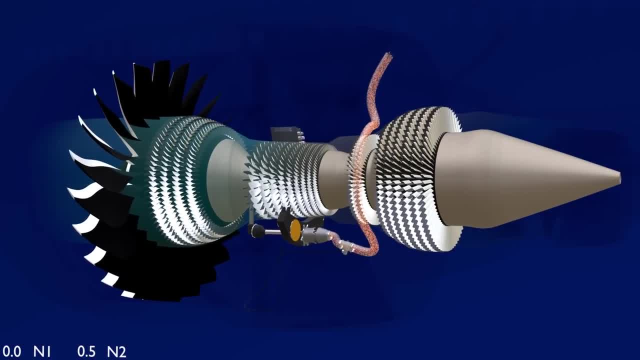 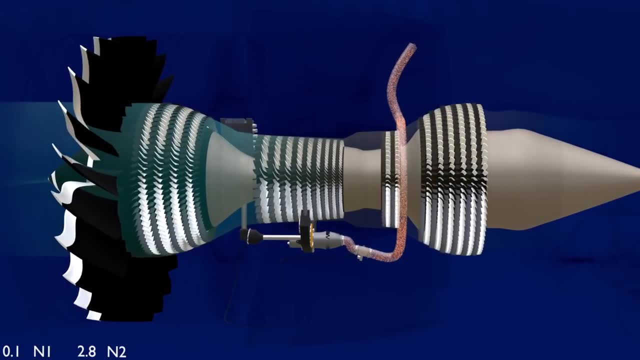 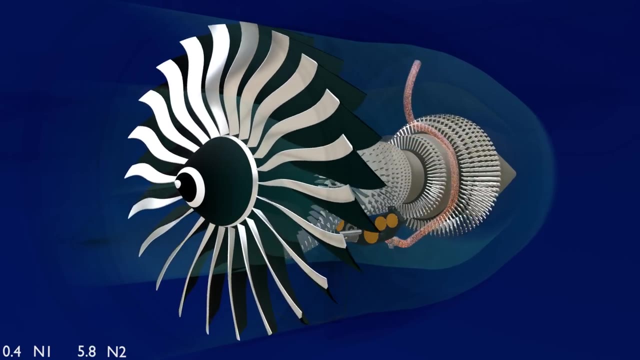 As N2 rises, airflow is established through the core of the engine. Due to the airflow, N1 shaft has positive rotation. Fan rotation in turn leads to bypass airflow through the engine At 7% N2,. a small alternator installed on the gearbox supplies power to the EEC. 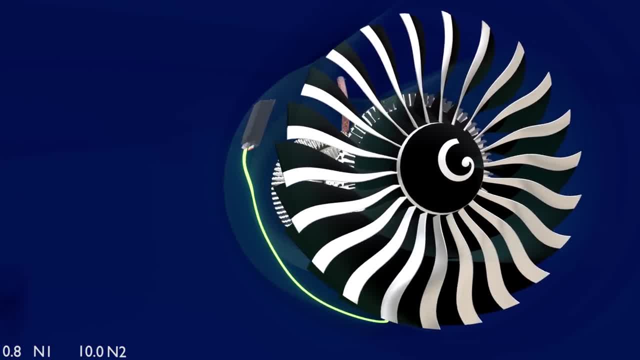 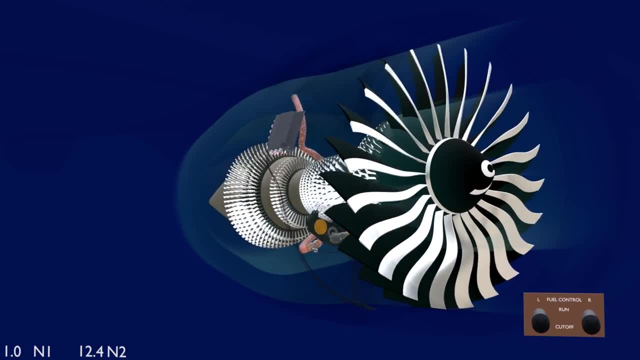 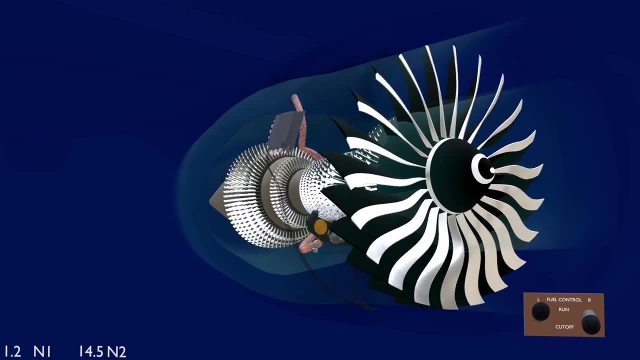 And the airplane power supply goes into standby mode. Since we are doing an auto start, we can use the fuel control switch and need not wait for the engine to reach 21% N2, which is the case in manual start. Let's select the fuel control switch to run and see how the fuel travels within the engine. 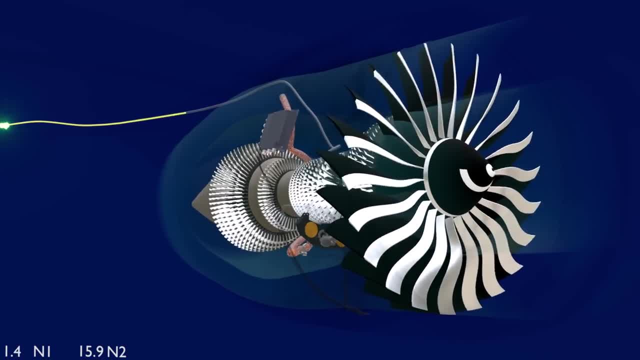 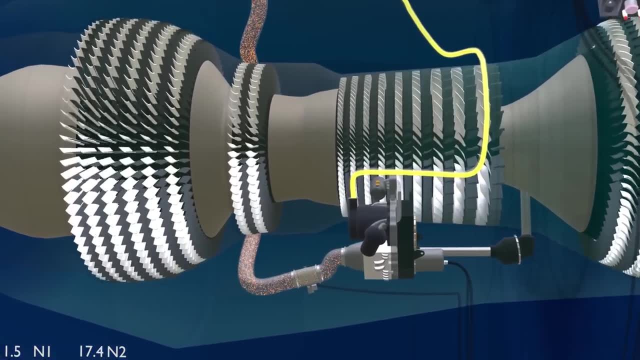 The fuel control switch opens the spar valve and the fuel rushes to the main fuel pump. The pump, driven by the gearbox, increases the fuel pressure and transfers it to the fuel oil heat exchanger, where fuel picks up heat and cools down the engine oil. 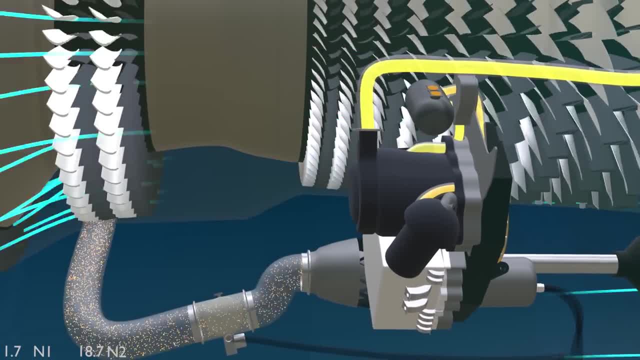 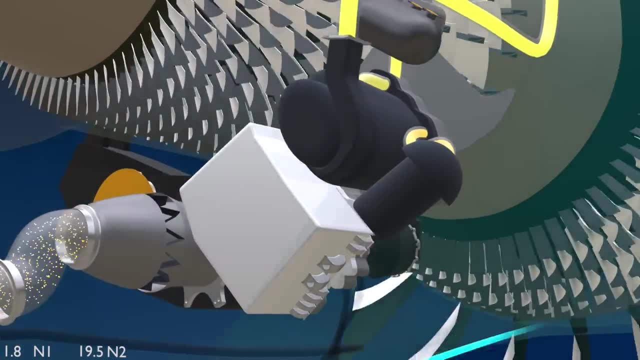 From the heat exchanger, fuel travels to the fuel filter. filter screens the fuel for debris and transfers it back to the pump. From here the fuel is sent to the hydro mechanical unit. The HMU now controls the fuel to the engine for combustion. 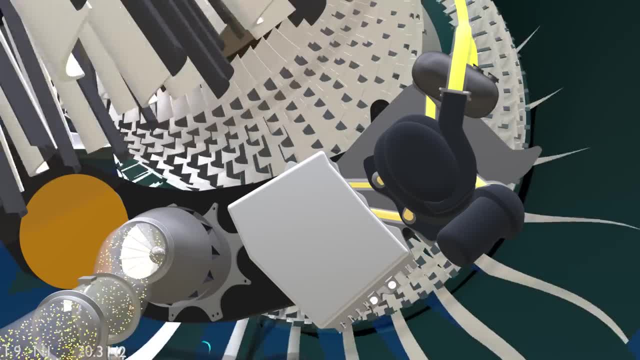 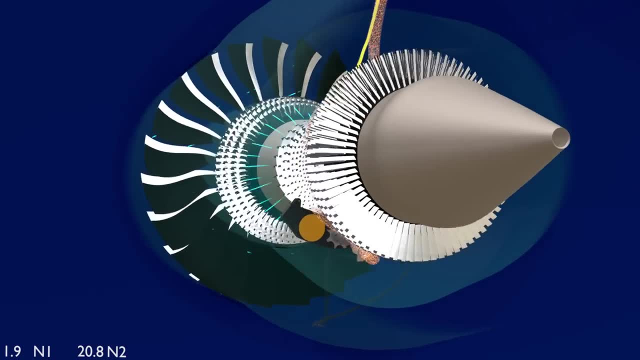 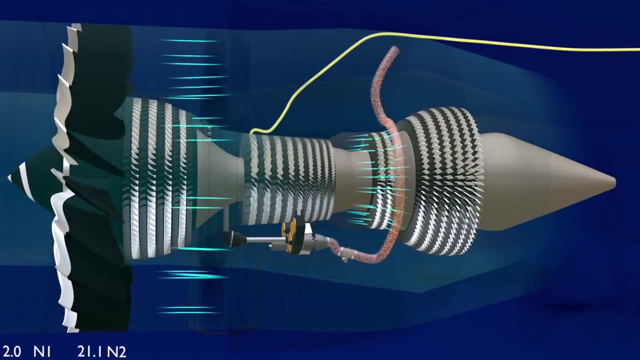 And any excess fuel is bypassed back to the pump. HMU waits for the EEC command to open the fuel shutoff valve And EEC waits for N2 to reach 21%. As N2 reaches 21% RPM, EEC sets up the engine for combustion. 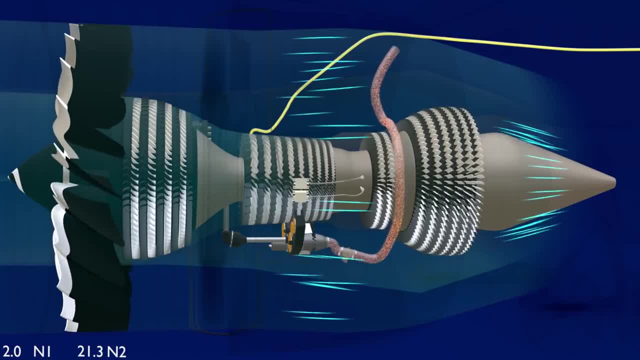 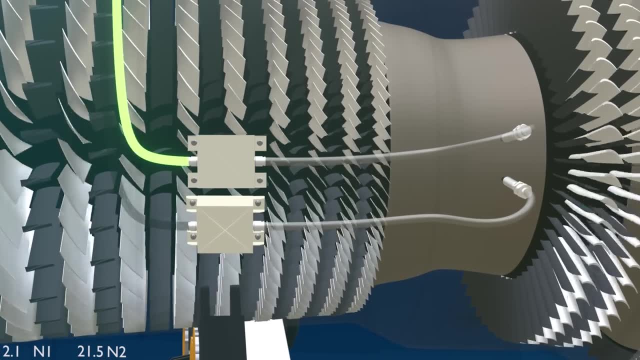 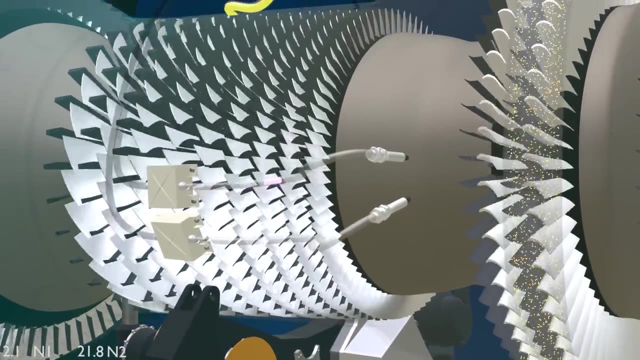 Out of two ignition exciters, EEC commands one to activate, keeping the other as backup. The ignition exciter converts the input power to high voltage pulse and transfers it to the igniter plug. Three seconds after ignition activation, EEC commands the HMU.